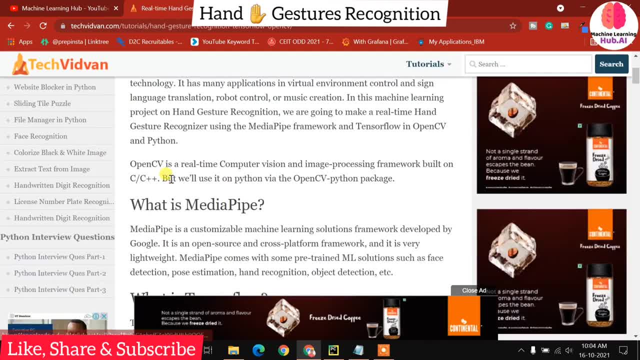 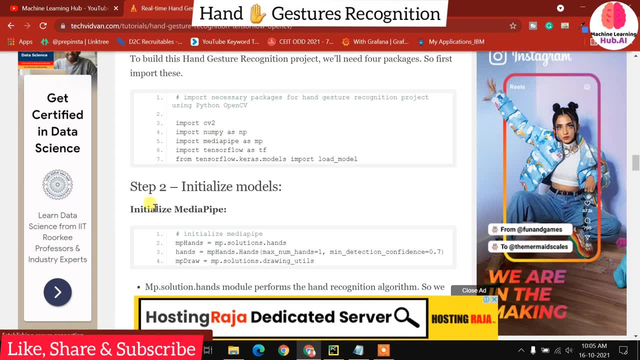 And you will get this code into this blog. You can see you can download the blog Code from here. This blog already link is given. You can see here you can download the code. So I am just explaining how you can implement this project. 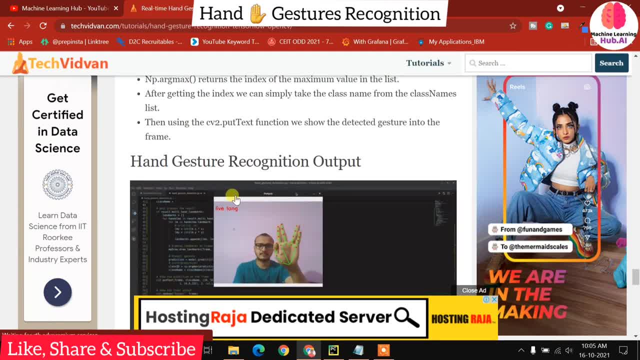 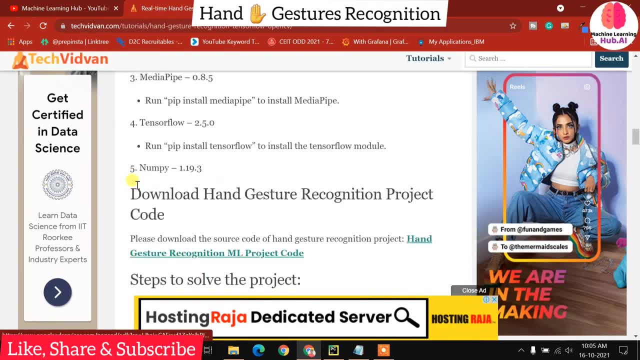 How you can setup the project and you can make this project running Even. you can see the demo is given into here. You can see. this is the summary and all the things are explained here. So we are just going to, And the first step is you just need to download the code from here. 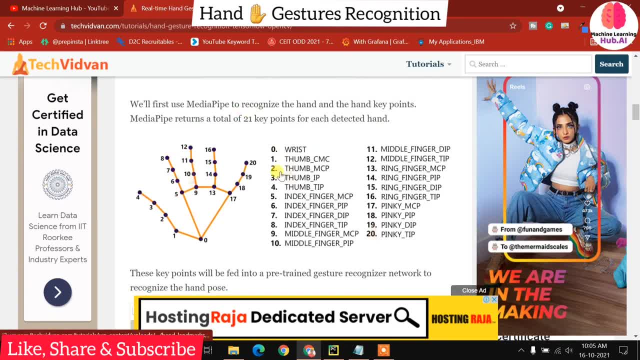 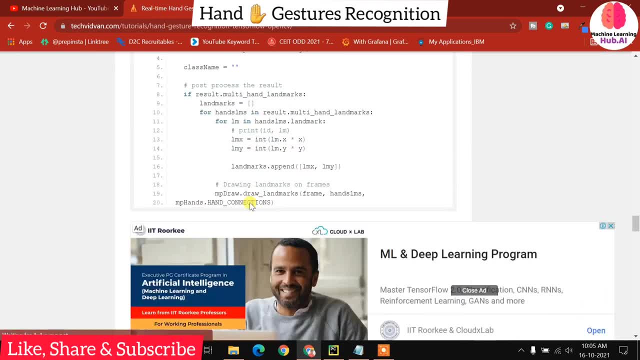 You can just read all the explanation and all the like Dependencies. all the things are mentioned here So you can read all. go through the blog. You will get the idea how it is working. In this video I am also explaining the same, So let's see. 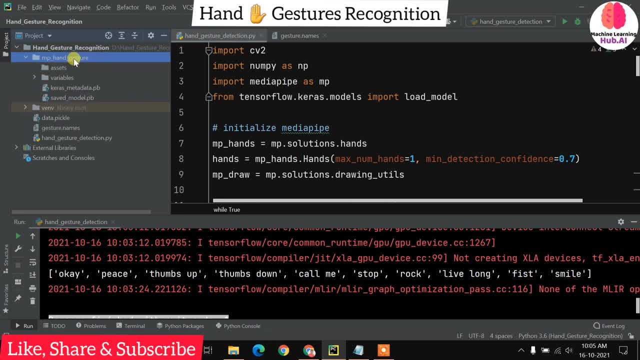 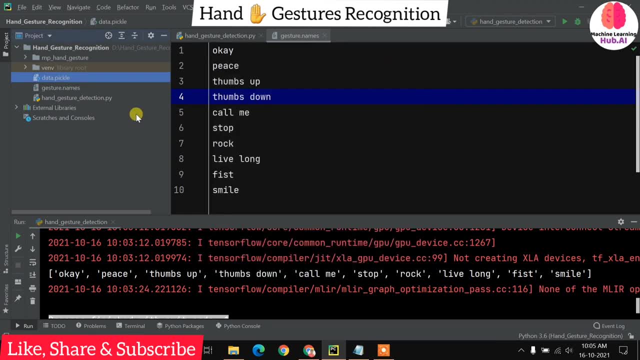 So when you download the code, you will get these things like MP hand gesture. You will get one code, You will get these names and you will get the data dot pickle file. So this is the structure of the project. So I just assume that you have downloaded the project. 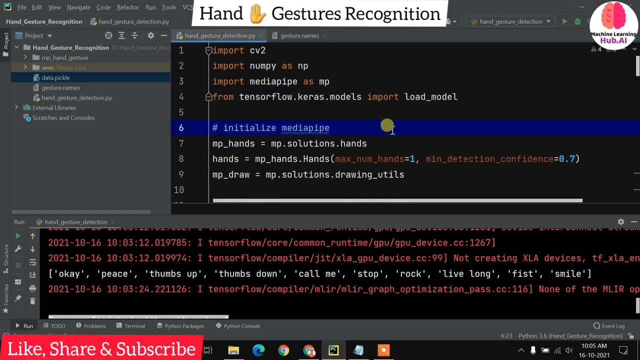 Now this project requirement is what? First of all, you should have the open CV, like CV2.. Numpy, Media pipe And tensor flow. Now, what is media pipe? I think all of you have listened: the Keras and tensor flow, But what is media pipe? 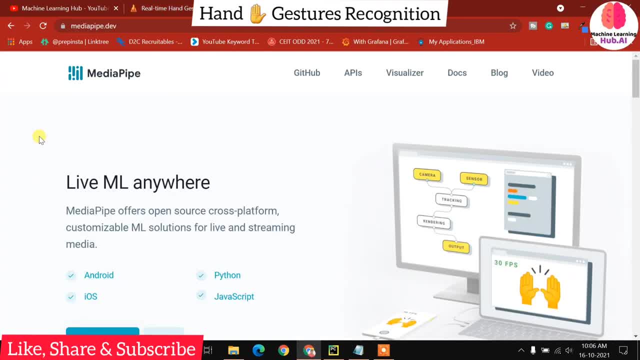 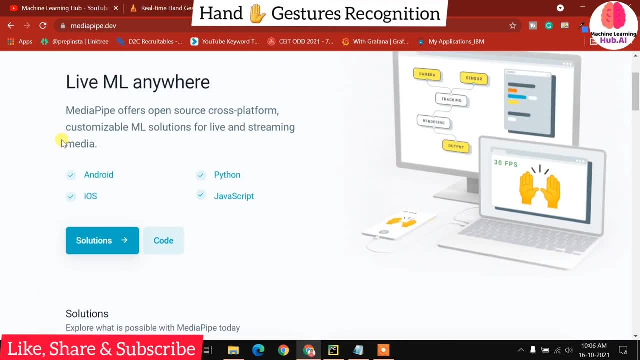 So let's see, We are going through this media pipe development site. So this is the media pipe. Now, what is media pipe is providing? Media pipe is first of all developed by Google, Which is providing you the transfer learning model, Which is already built. 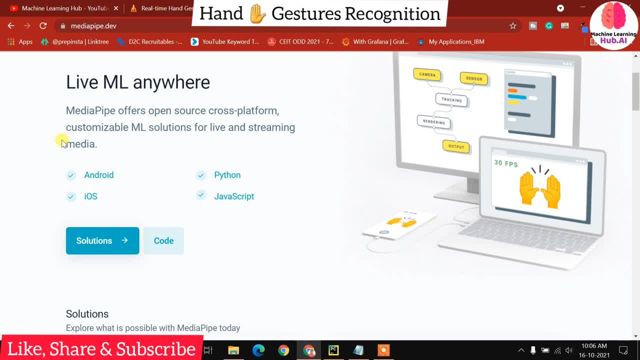 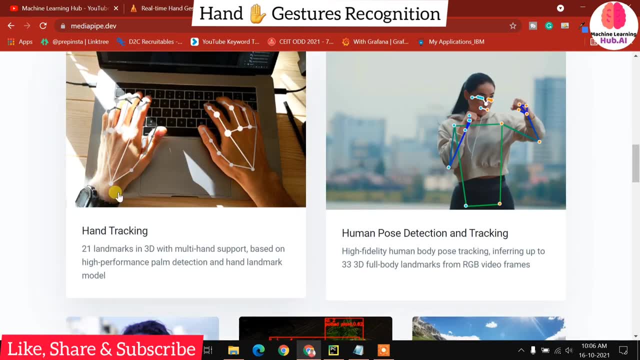 And you can see. it is very like open source And you can create a. That means application You can see, like selfie segmentation, Face mesh- All the things are open source. You will get a ready made, pre trained model And you can implement your model into your android application. 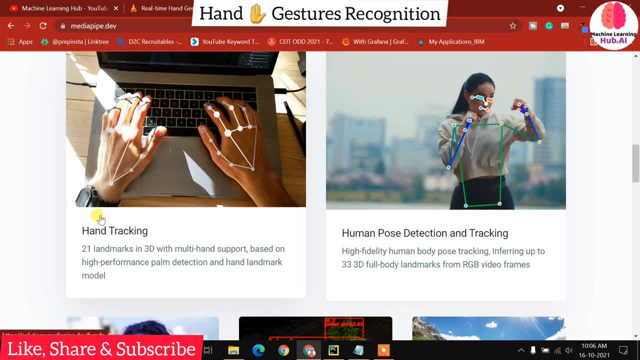 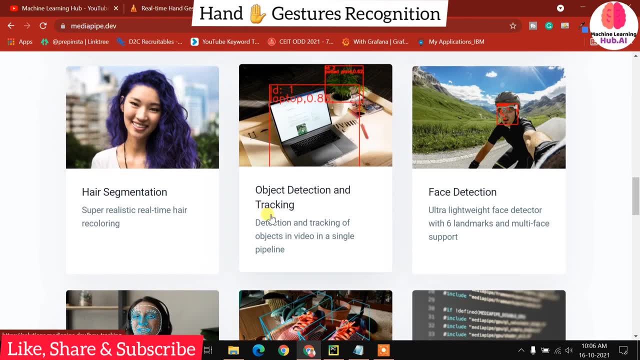 Means. you can create a cross platform application. So this is like you can see in this: human pose estimation, Hair segmentation. So all these thing and all the models are open source. You will just use it And you can deploy this thing into your application. 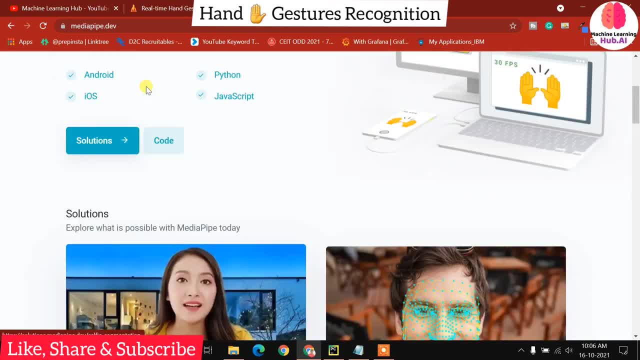 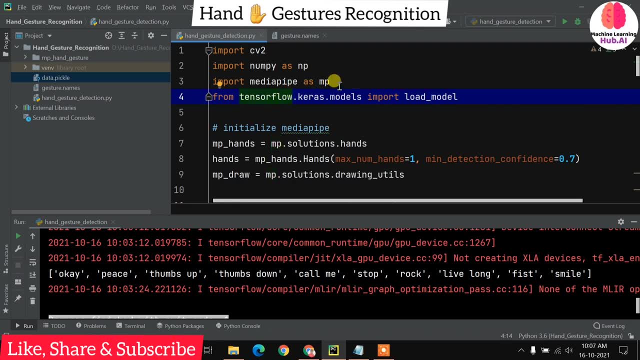 So this is the main thing you need to about see this media pipe. So we are using pre trained model. We are using pre trained model from media pipe, So we just need to use media pipe, For in this project we are using media pipe. 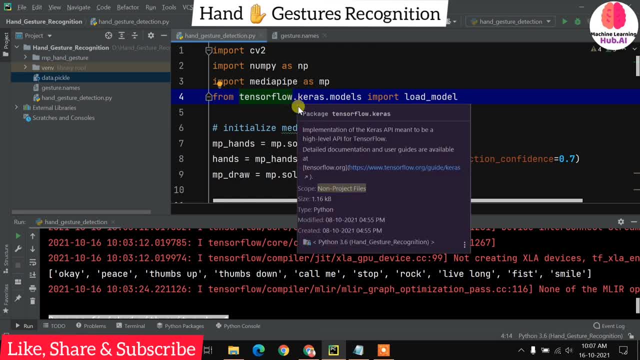 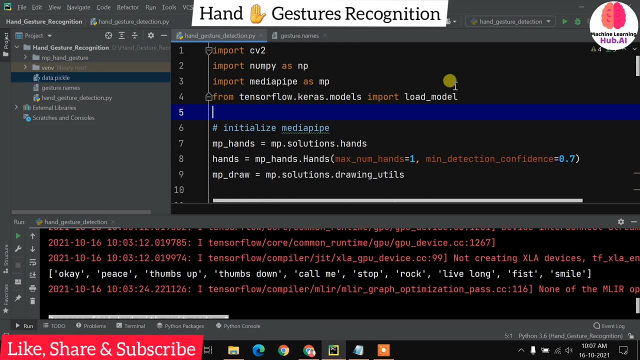 Just for detecting the hand movement Right Now. the another one is tensor flow. Now we are using tensor flow for predicting the movement. Just understand the difference. Media pipe is just for the detecting the movement, But tensor flow for predicting the hand movement. 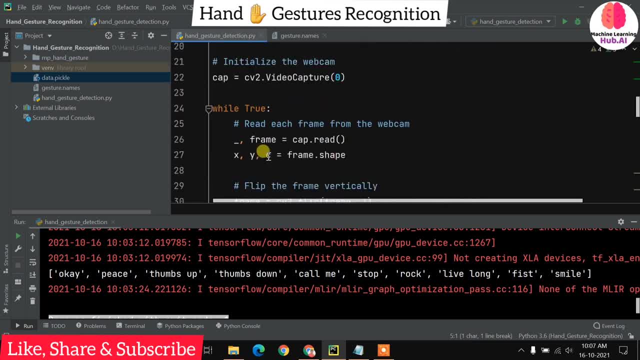 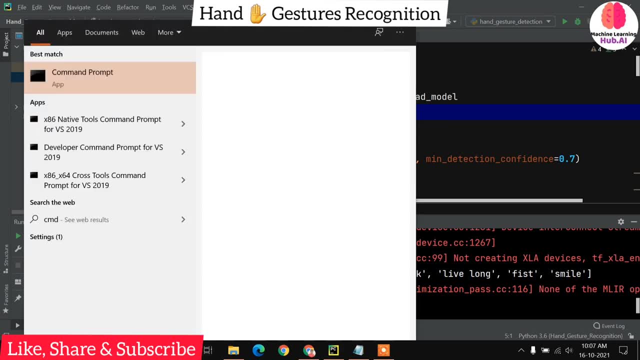 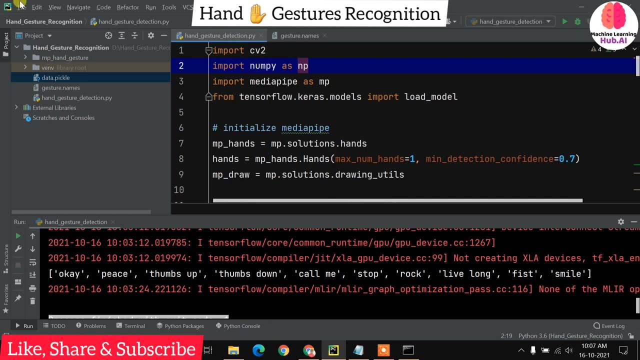 So now let's see how we are going through this code. Ok, So now, first of all, we just need to import all this thing. So if you have not installed this library, Then just go to command prompt. You just need to do pip, install, media, pipe, open, cv, hyphen, python, then numpy and tensor flow. 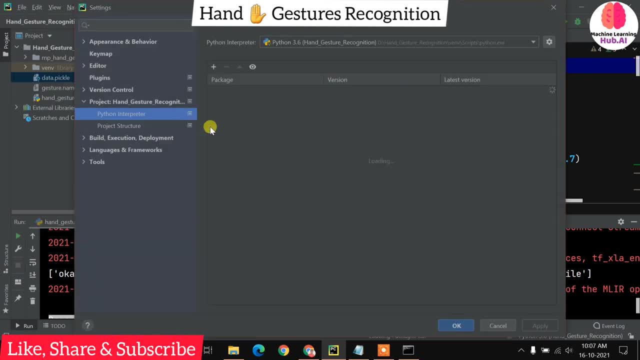 If you want to check the version, then let me show you the version of media pipe and all Ok. So which version of media pipe I am using? 0.8.3.. Let's check it for the tensor flow. So ok, I am using 2.4.1 tensor flow. 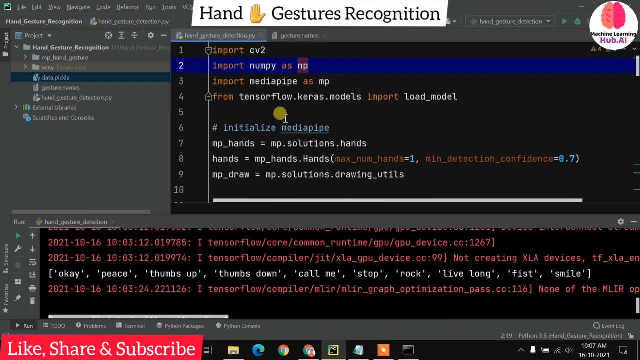 So you will get this version. This is running fine into my system. You just need to import Means. this code is already given. You just need to understand how this is working. So now, first of all, we need to initialize the media pipe. 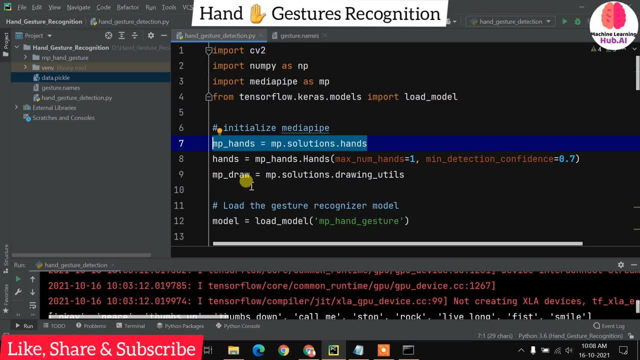 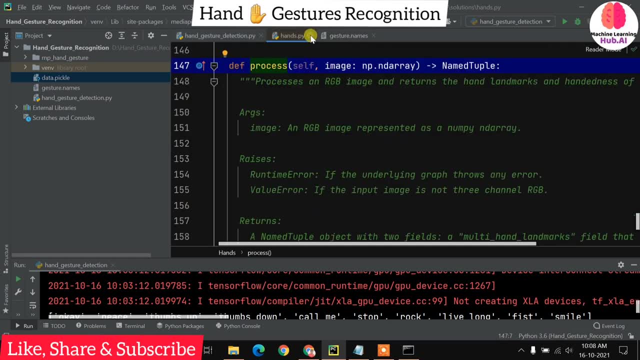 Because we are going to use it. So mp underscore hands is equal to mp dot solution dot hands. So basically what we are doing, We are implementing the hand detection algorithm Here. you can see hands dot py. So this is the algorithm. Now we are tuning the algorithm. 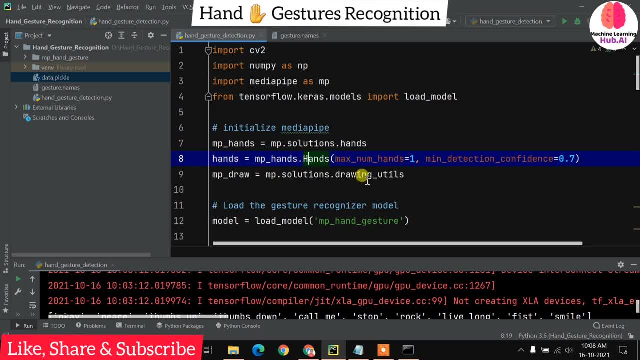 You can see mp hands, dot hands Like maximum number of the hands. So in this, just in this project, We are only detecting one hand at a time And minimum detection confidence is 0.7.. So you can change this confidence Confidentially according to your like. you can put 0.567.. 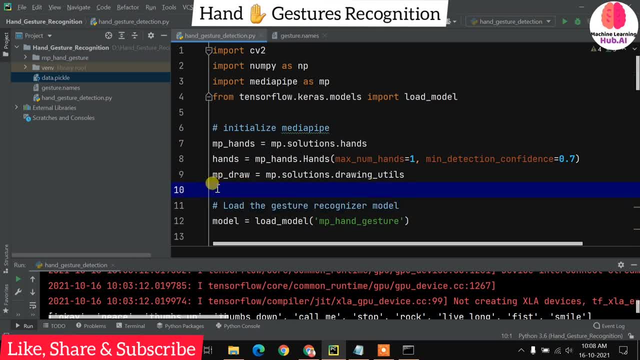 According to your, Now we are, We need to draw the hand movement onto your system, Right? So mp underscore draw is equal to mp dot solution drawing utils. So basically, this is just simple, like what we are doing in open cv, Like cv2 dot rectangle, cv2 dot text. 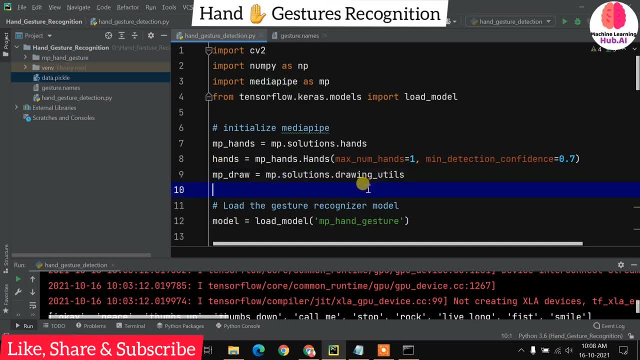 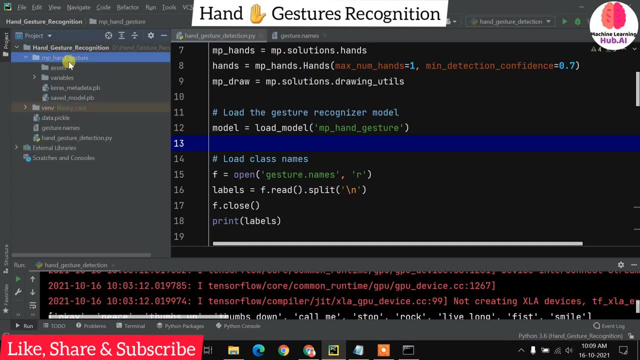 Means you can, How you can put the text and rectangles and you into into your frame. So this is a simply drawing utility. Now we need to load the model and this is the model So you can see the. in this model folder You will get a pb file of the keras and assets. 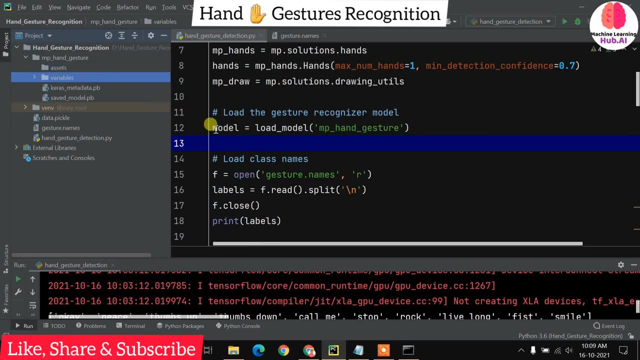 You will get like variables. You can see these. all are the approaches. Okay, So we need to this more. load the full folder. You can see mp underscore: hands, dot gesture. So we need to load the full folder into this model. Now there is a one list here which is containing: 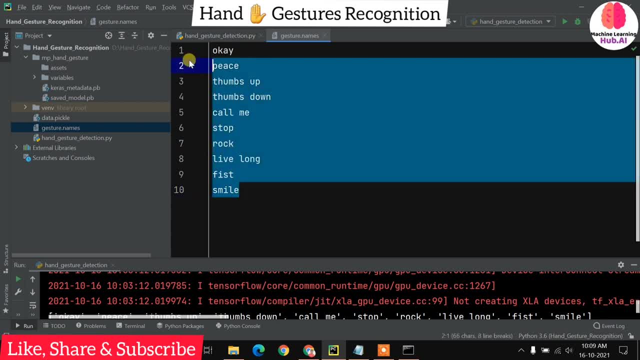 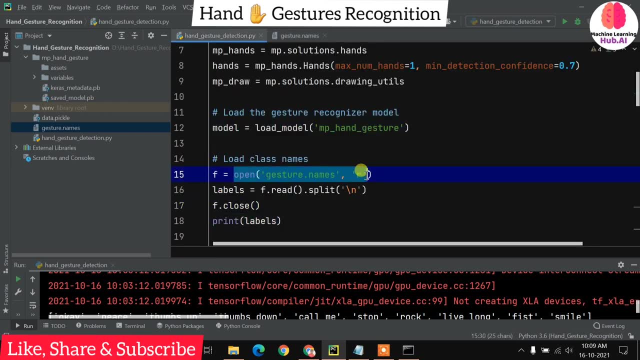 Only the kind of the not profile. You can see this only contains the name of the gestures. So we need to read that file also like f dot open. Basically we are just using the file function gesture dot names, We are reading it and then we are just splitting with this lesson. 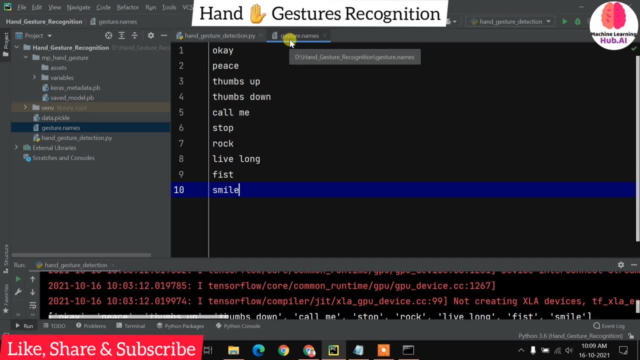 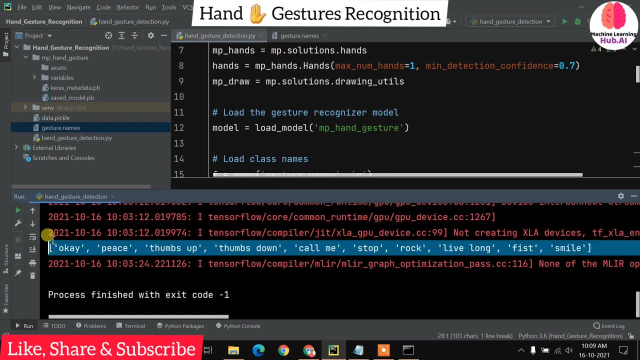 Lesson just means what by which is splitting with the enter only. So what we will get? we will get this kind of the ready-made list here. Okay, So you will get this ready-made list. So basically we can classify the result and we are just printing the label. 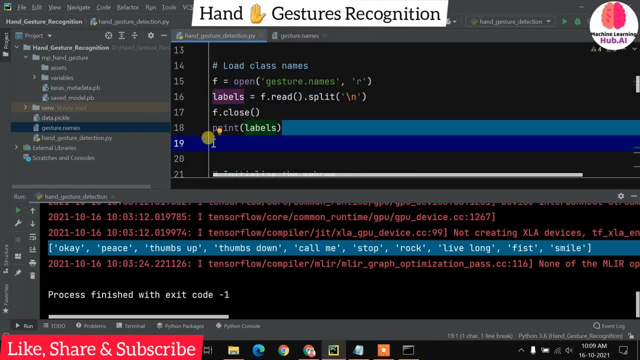 Okay, So this is. this is basically our labels of the recognition. Now, this is the main part. start from here. Initialize the web cam. So cv2 dot, video capture zero. So if you have external webcam, you can use the one here. If you have any kind of the cctv webcam, 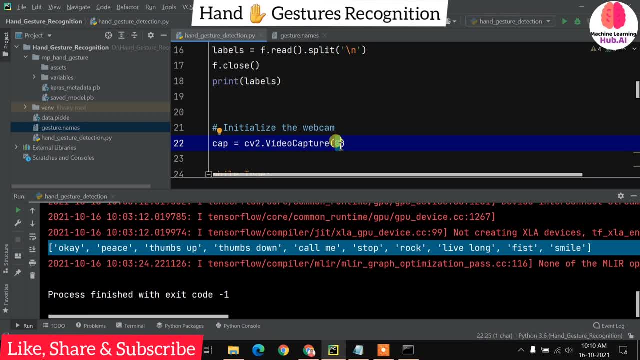 If you want to any use cam, Then you just need to put your url here Right now. while true, because we are playing with the frame, We just need to go into the infinite wild route. Now we just need to read the frame like that: 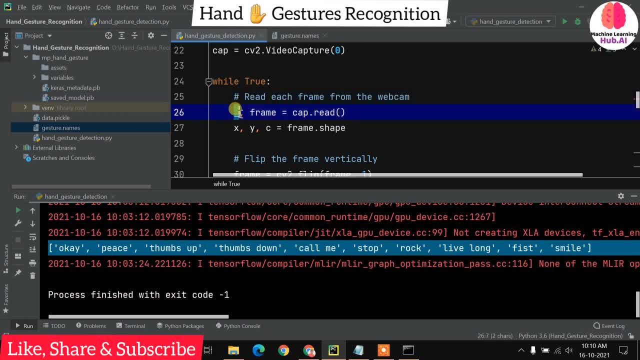 like cap dot read now this or this underscore and this frame. so basically cap dot read. return a two values: one is the frame and one one is the boolean like true or false. if you are getting the frame, then it will be true, otherwise it will be false. now we are just checking the shape, like x. 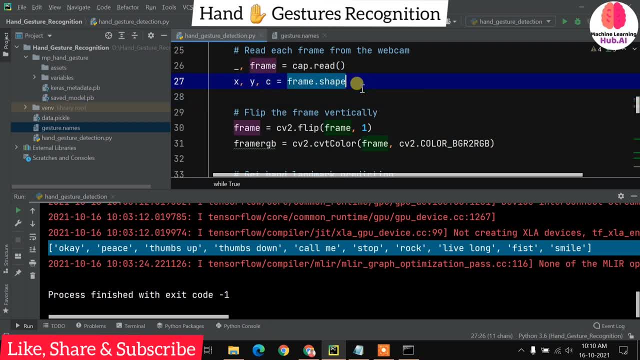 comma y dot c. y comma c is equal to frame dot shape. now what we need to do, flip the frame vertically like frame is equal to cv2 dot flip. and we are just flipping the camera right now. we need to understand one thing here: what we are doing is frame. rgb is equal to cv2 dot, cvt color. 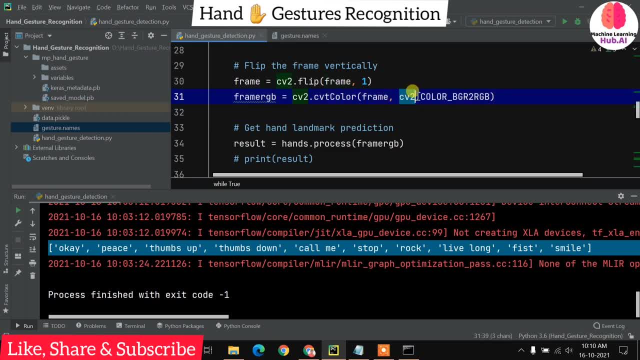 and then we are changing the color format of the our frame because always remember cv2, always working with the bgr format, right, but if we want to do anything, then we just need to like, if you are playing with any images like we are doing it- skm or pil or anything we need to convert into. 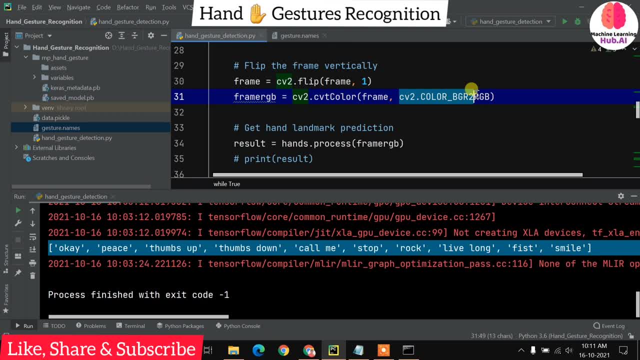 rgb but always opens. we work with the bgr format, so we need to convert this frame into bgr to rgb. right, because this algorithm is work with the always. obviously it is rgb, so we need to convert the frame before it. now get the hand landmark: landmark prediction. you can see result is equal to hands dot process. now we are. 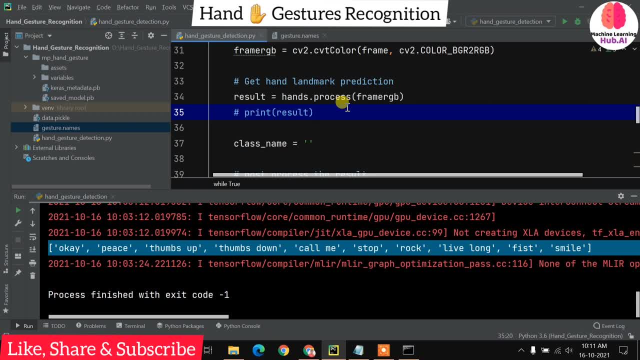 processing the frame, we need to find the hand from the frame, right. so we just need to pass this rgb frame into our algorithm, which is hands dot process. now we just need to initialize the class name- just empty variable to give the proper hand movement name. now, if result dot multi, landmark this. 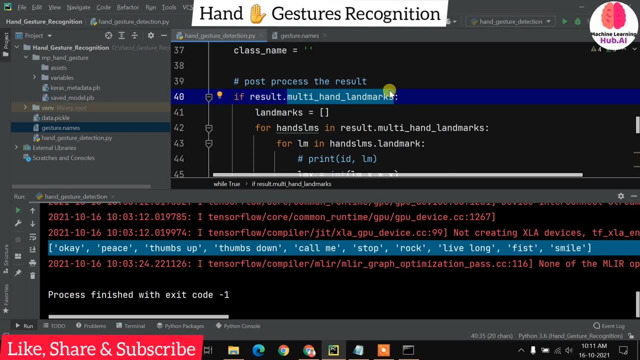 is the hand is detected. so with this method, we will know means if any of the hand is detected. if not, then it will. it will, uh, don't show anything on the frame, but if your hand is detected from the frame, right. so what it will do. we are just creating the landmark list, empty list. i will explain it. 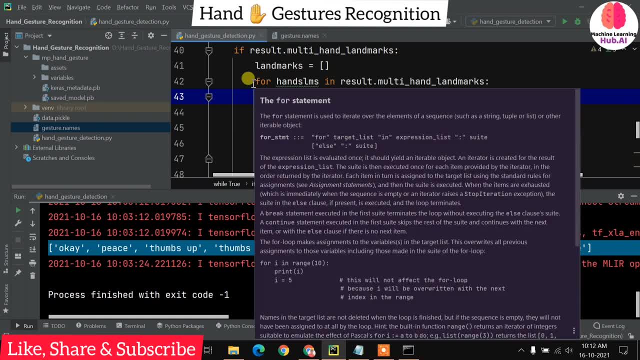 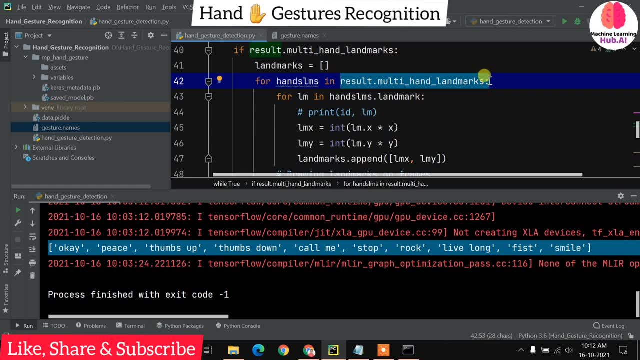 later why we are creating the list now for a hand: lms in result dot, multi landmark, what it will do when the hand is detected. if the hand is detected, you can see the multiple times of the hand is of the means multiple uh points are detected for. so what we are doing? we are iterating each 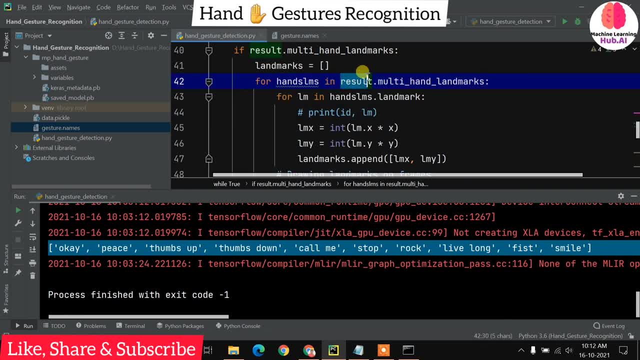 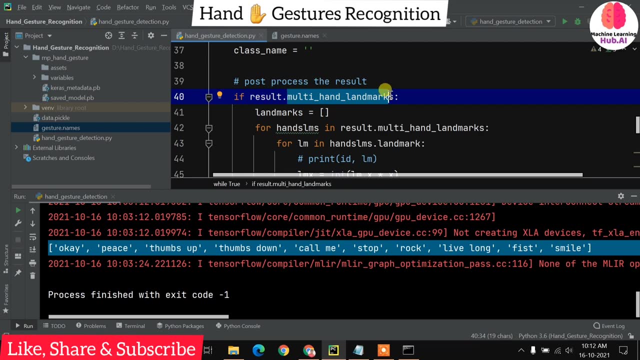 point and if in result means what we are doing. if result is detected. detected, we are iterating to each points and multi hand landmark. you can see we are using the same method again. if it is detecting means if the hand is detected, we will go through the whole, the whole uh points. 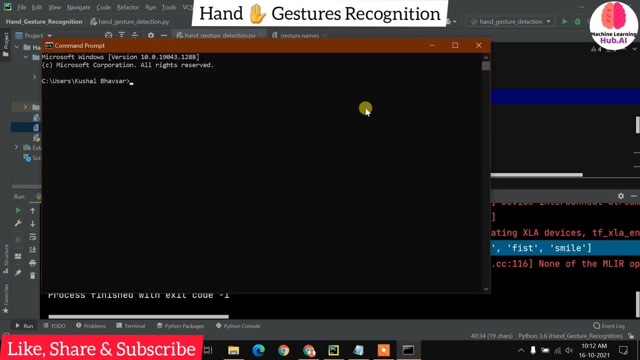 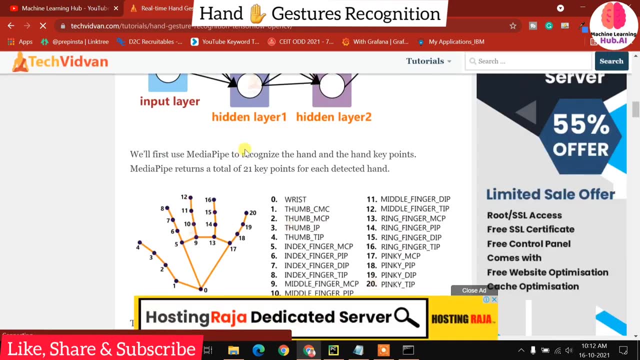 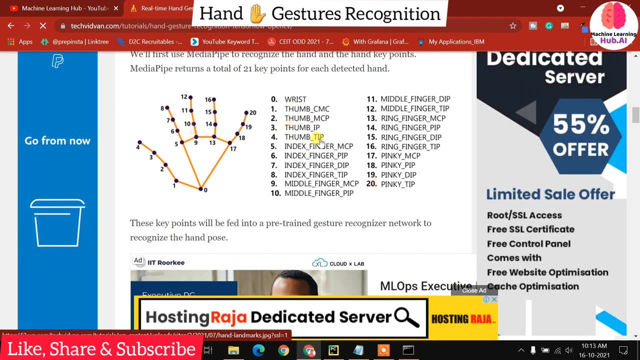 of the bunch, you will get a you. if you have not observed, just let me show you the example here, uh, you can see, here, uh, there is a one picture of hands. okay, so you can see. these all are the points you can see. zero is raised, one for the thumbs. so it will go through each point, right? so that's why we're using 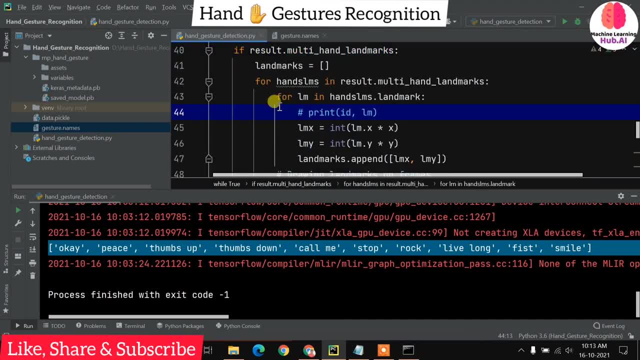 the fall of here. now we need to store the uh hand landmark right. we just need to store the height and width. you can see lmx is equal to integer. so what we are actually doing here in lmx and lmy, we are storing the our coordinates right. 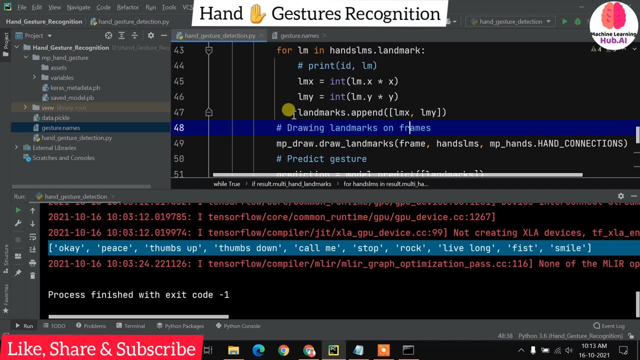 like width and height. now we are appending this thing into landmarks, so landmarks dot append, so that's why we have created the implicit here. so this is the reason, right now, what we need to do. we have detected our hand movements. right, you can see these. all things are detected, but the 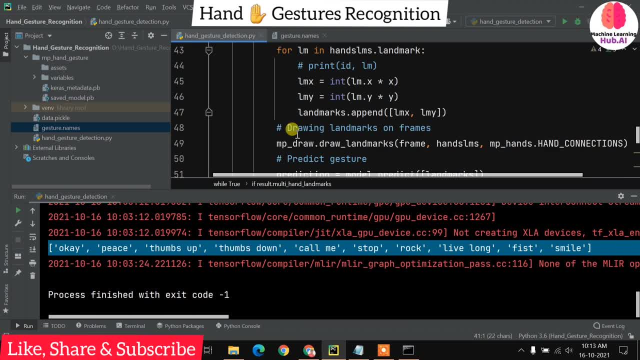 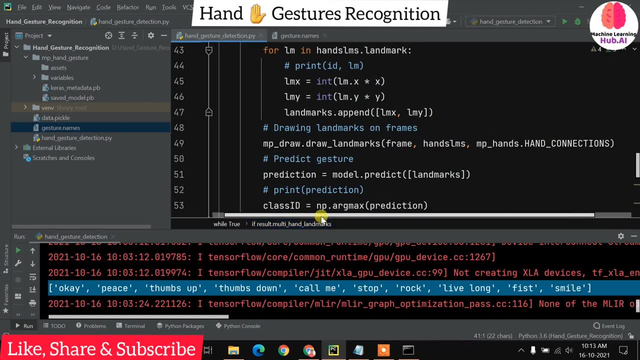 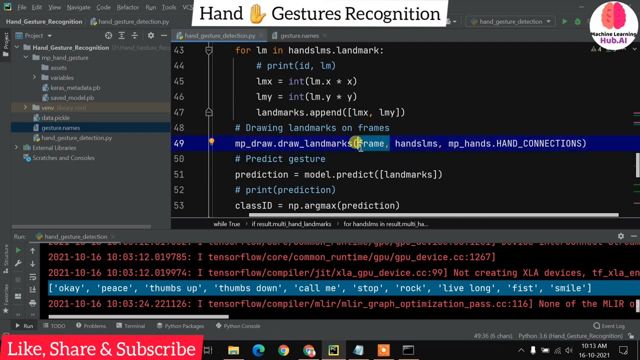 main thing is to draw this thing into our real time frame. so what we are doing, mp draw already we have initialized our drawing method here, so mp draw, dot draw landmark right. so one which frame we need to do on the our original frame, right, it is bgr frame, it is not rgb, remember that. 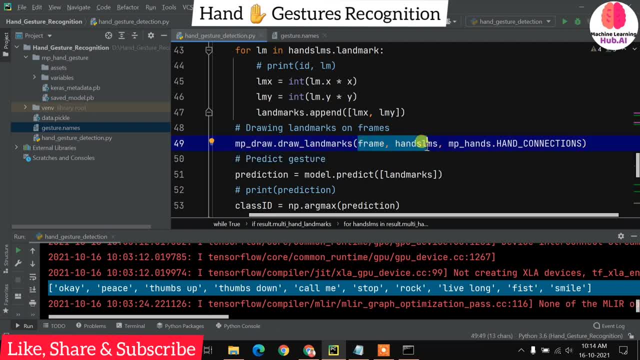 on to real frame. we just need to draw all the things and we can. what we are doing in hand lms, we are passing this hand lms, then mp hands and then hand connection. so basically what we are doing. it will give you the connection. like this you can see. all the points are connected. 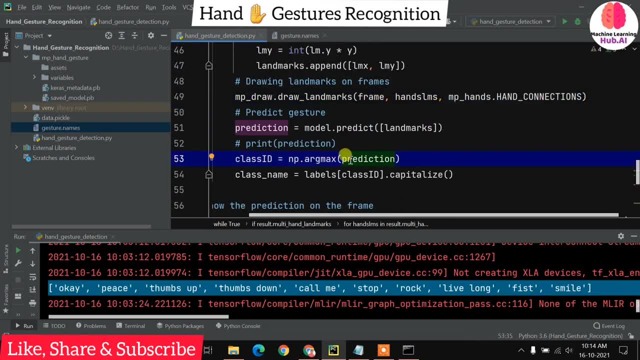 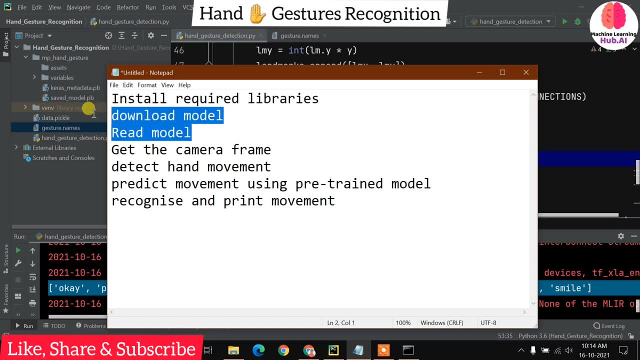 here right now, our first task is completed. right, what we have done? first of all, we have all the required libraries, we have downloaded the model, we have read the model, we will just load the label, we are getting the frames and now our uh one uh task is completed, which is: 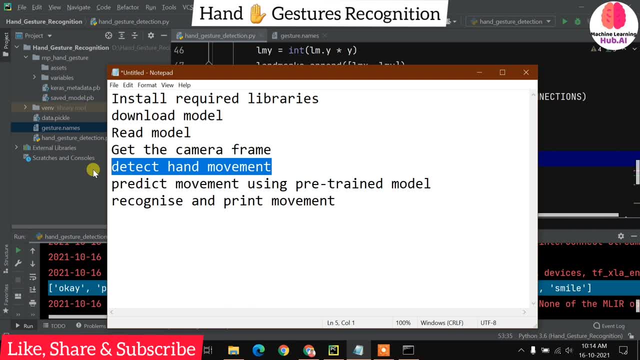 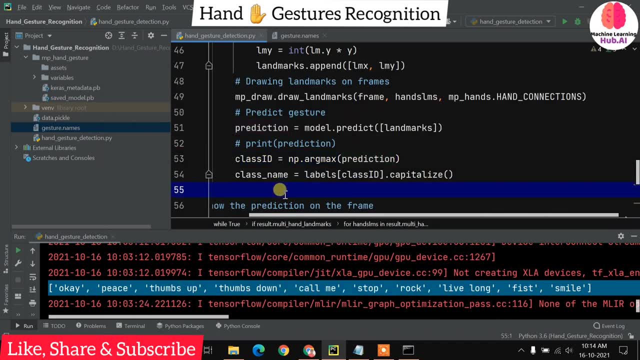 detect hand movement. now our hand movement detection is completed. now what we need to do? we need to predict this hand movement, like what i am doing. i am doing a gesture, which kind of the gesture, right? so what we need to do? prediction is equal to model dot. predict now in model dot. 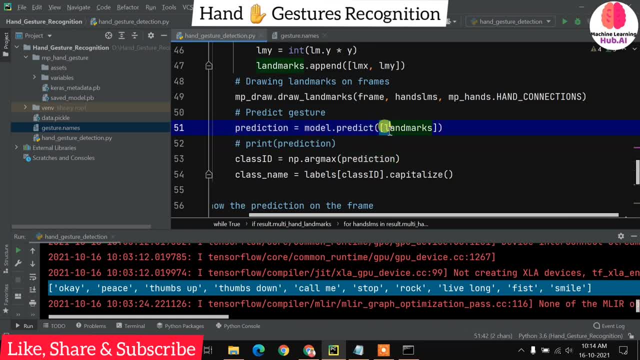 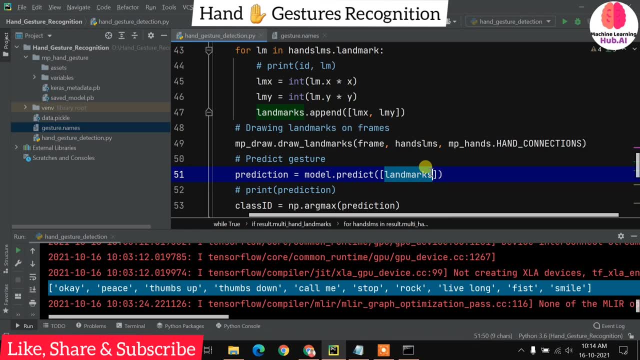 predict in parameter. what i have passed is one list into one list. i am passing another list of this landmark. that's why we have created this list, so in two lists i am passing the list so you can understand how this concept, if you are, if you know, if you pass only this one list, you will get. 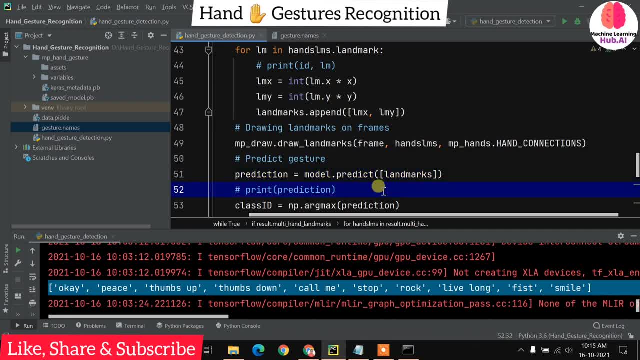 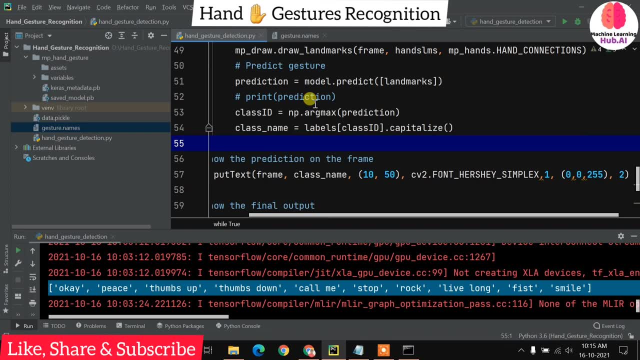 the error. so at least into list we are passing and what we are doing. this prediction will give you the uh kind of the prediction like you will get the labels like 0, 1, but now what we need to do, you will get a lots of big error right. so we just need to get the np dot argument max. so what it will do. 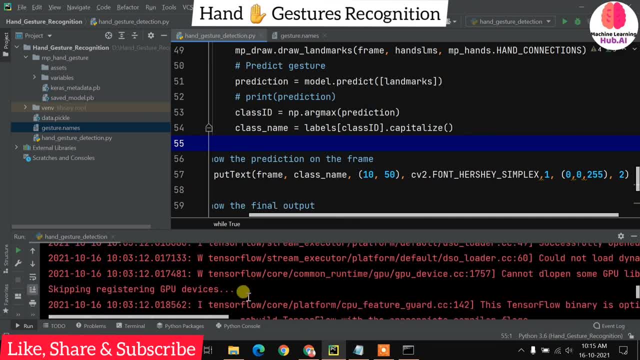 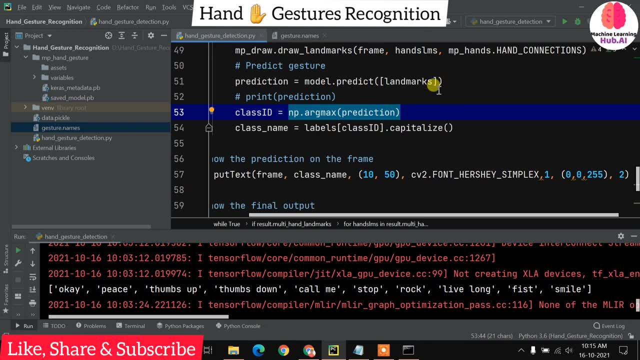 uh like 0, 1, 2, 3. you will get like this. you will class like uh 4. okay, you will get 0, 4, ps. you will get 1, 2, 3, right. so with this np arguments we can do this like: right now we need to find the prop: uh, proper class name for our. 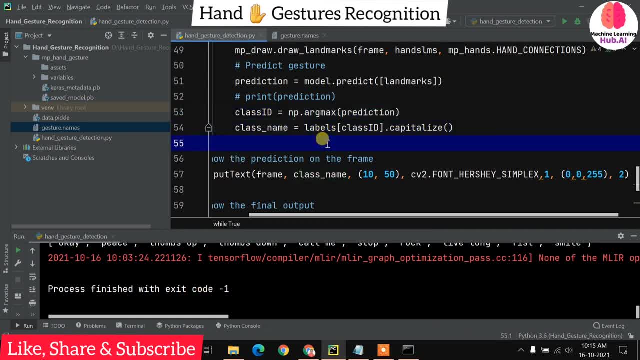 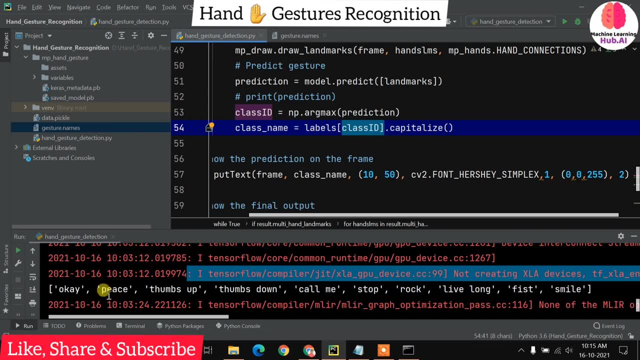 moment. so what we are doing: class name is equal to labels, labels. already we have initialized: this is our labels, and then labels dot class id. so class id will be like 0, 1 if i am doing the sign of the piece right. so what? i will get a class id. i will get one, and for a one, obviously it is pcr. 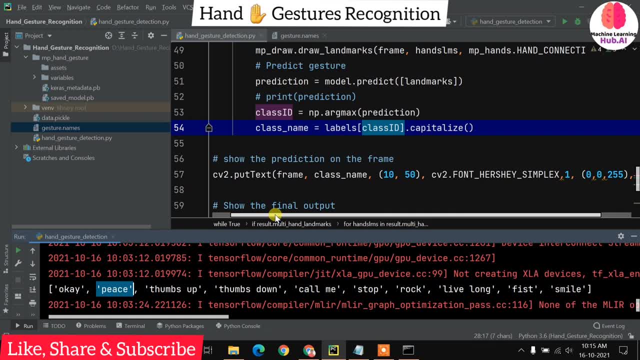 i will get the perfect label name from the labels for the particular moment. now i am just doing capitalize because it is written in small. so this is just kind for the good looking purpose. now what i am doing: i need to put this result on the mainframe so for cv2, dot put text what i am doing. 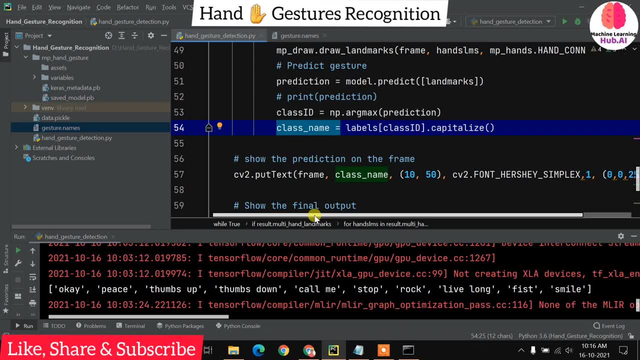 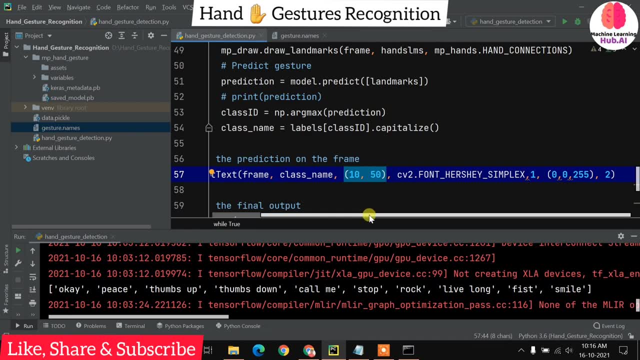 is. i am just putting this label into frame, so frame you can see. these all are the like 10 and 50, like x is like height and width or not. it is not height and width, it is pixel, like x and y. you can understand, like, if you just assume the graph now, then cv2.4 hashes simplex. i'm just uh passing the. 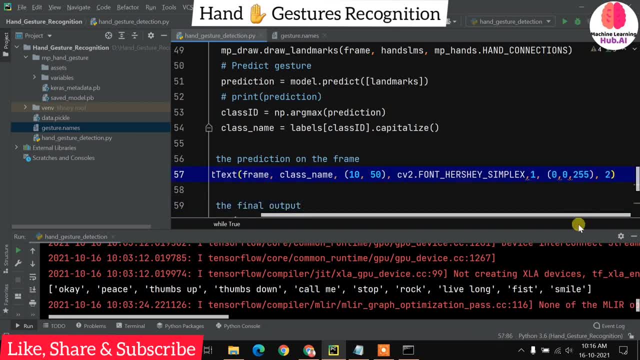 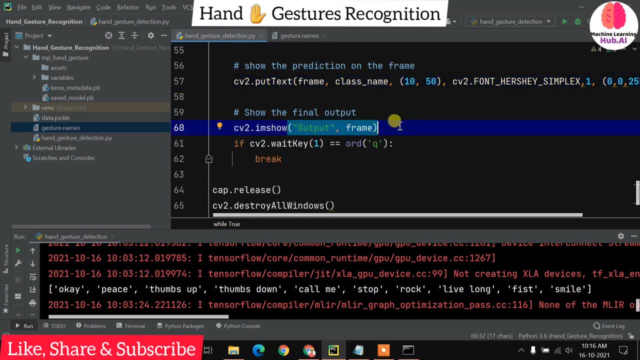 red color like zero, zero, two, five, five. i'm just passing the rgb and this two is the width. uh means height bit and we can say we top the, our font now, cv2.i am sure output. i'm just uh showing the result frame if weight, k and order humans. if i am pressing the q, then automatically my system means: 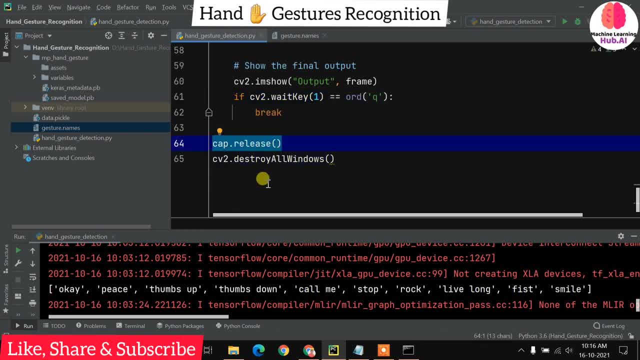 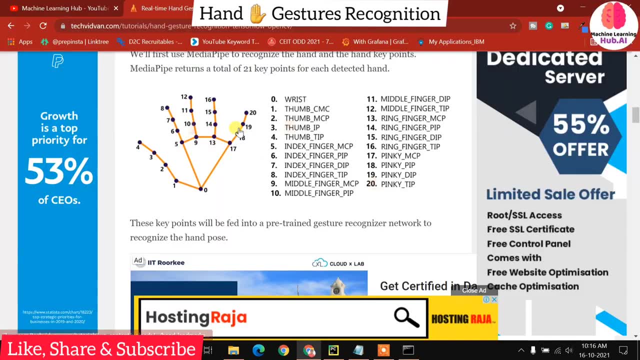 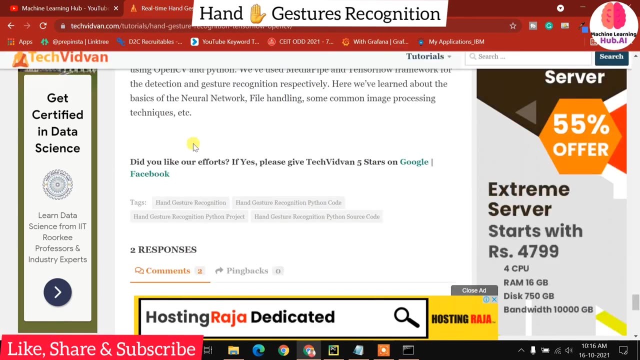 my frame will be closed and after that my cap means camera will be released and after all the windows will be destroyed. so i hope you get this code. even this explanation is given in this video also, i'm sorry, this article also, so if you want to read the written all the things, you will get this. 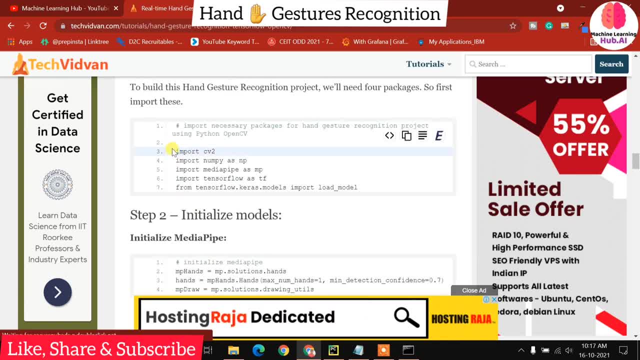 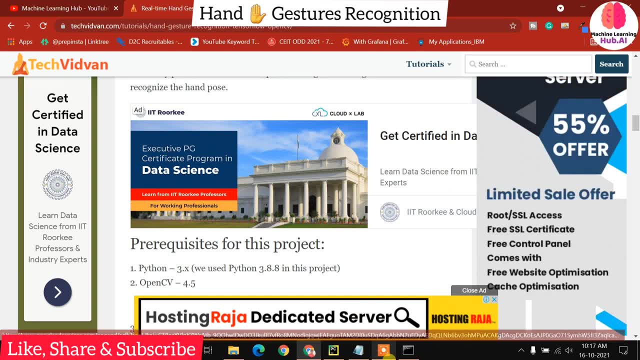 all the things here you can see. the code is, link is already here. you can download the code from here. and the beautiful you can see, the powerful explanation is also given here. right, you will get a perfect idea to explanation, right? so now we just, once again, we are checking the mover.